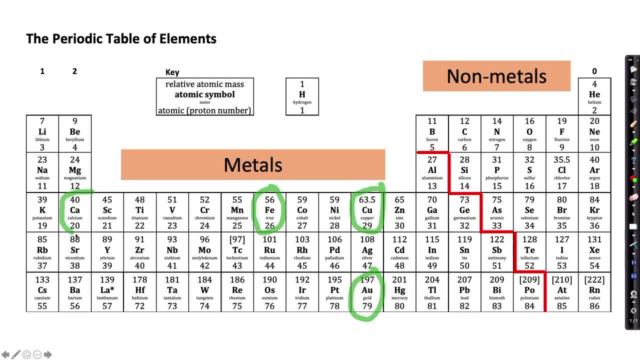 For example calcium, But all of these elements to the left of that red line have similar properties. On the right hand side are all the non-metals, For example oxygen and chlorine. Many of these are gases at room temperature, But you also have elements such as carbon. 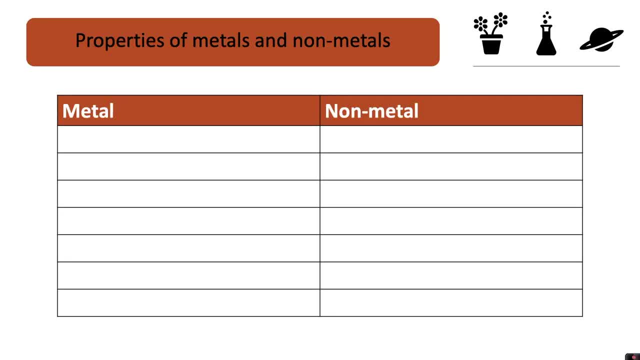 which are gases at room temperature, But you also have elements such as carbon, which are solid at room temperature. All of the metal elements have similar properties to each other And, in the same way, all of the non-metal elements have similar properties with each. 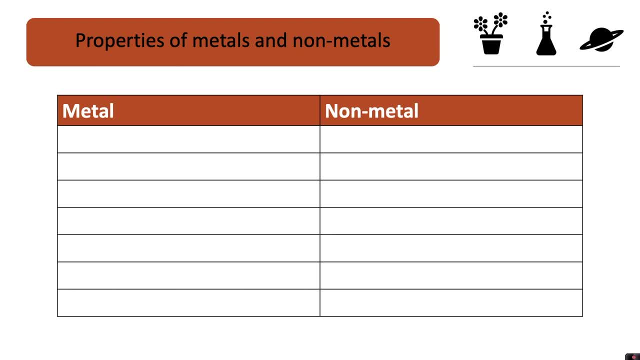 other. We're going to go through the general properties of metals and non-metals. Metals are shiny. Non-metals are dull. Metals are sonorous, which means they ring when they are hit. Non-metals are not sonorous. Metals are malleable. This means 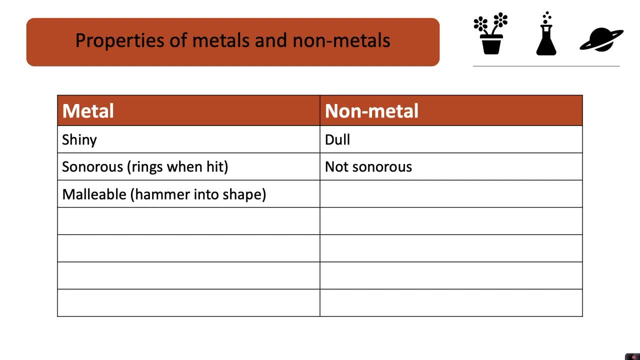 that you can hammer them into different shapes. However, non-metals are brittle. If you were to hammer a non-metal, it would just break apart. Metals are ductile, which means that they can be drawn into wires, But non-metals are not. Metals are ductile, which means that they can be drawn into wires, But non-metals are not. 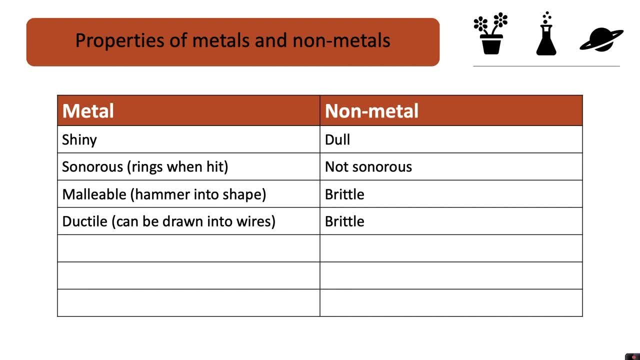 Metals are brittle. Again, these non-metals would just break apart, so you couldn't actually draw them into wires. Metals generally have a high density, whereas non-metals have a low density. Metals are good conductors of heat, whereas non-metals are not. And finally, 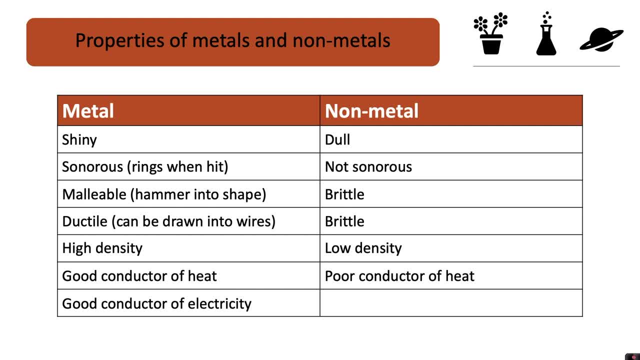 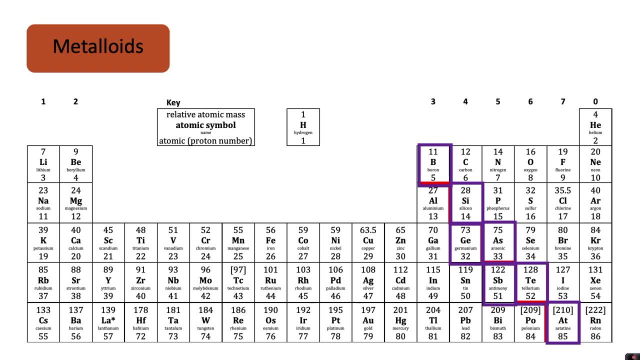 metals are generally good conductors of electricity. There are some elements that lie very close to the line that separates the metals and the non-metals, and we call these metalloids. Metalloids have properties that are in between that of metals and non-metals, So for these elements you might find that some of their 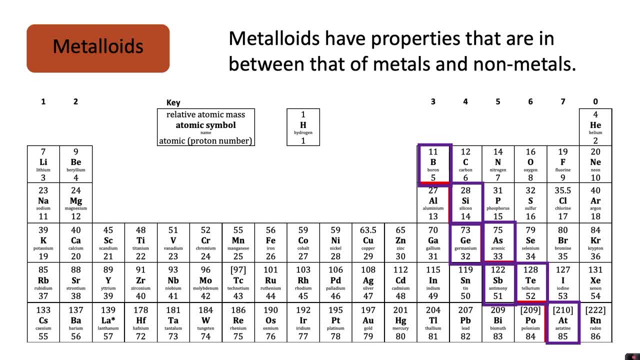 properties are very similar to metals and some of their properties are similar to non-metals. Both metals and non-metals are non-metals. Metalloids have properties that are in between non-metals and non-metals, So the non-metals may be non-metals, but they are also non-metals.